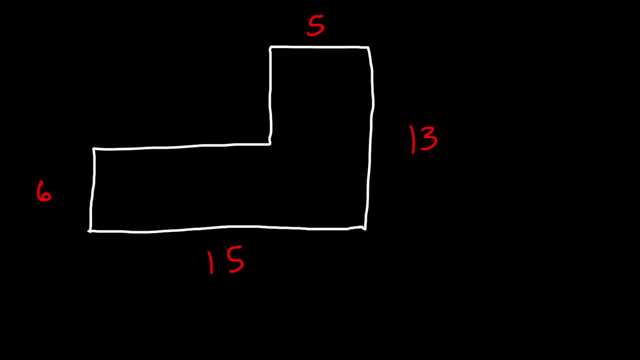 Using what you know, calculate the area of this composite figure. So feel free to pause the video and try it Now. what we need to do is break this area, break this figure, rather, into two rectangles. So I'm going to draw a line. 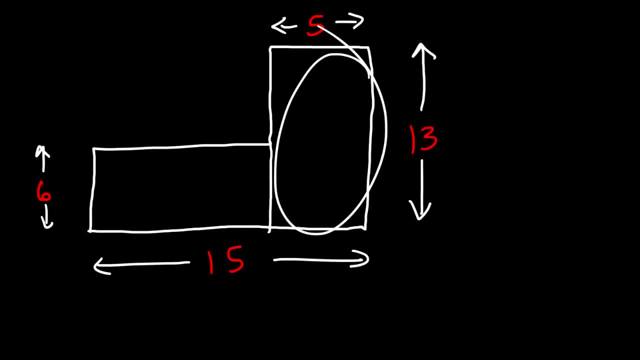 So what is the area of this rectangle? Well, it's going to be the length times the width. So 5 times 13 is 65.. Now, what's the area of this rectangle? Notice that this side is 15 and this side is 5.. 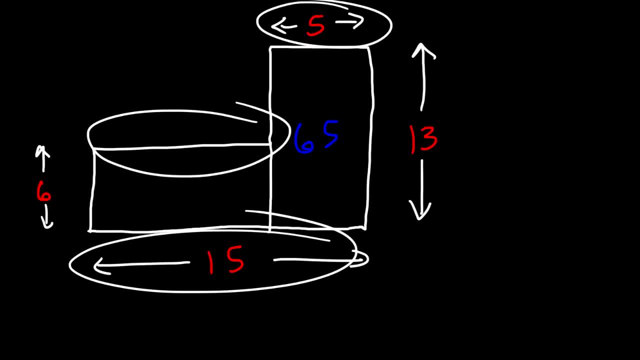 So this side has to be the difference between 15 and 5.. So 15 minus 5 is 10.. So this side is 10 units long. So this rectangle has a length of 10 and a width of 6.. 10 times 6 is. 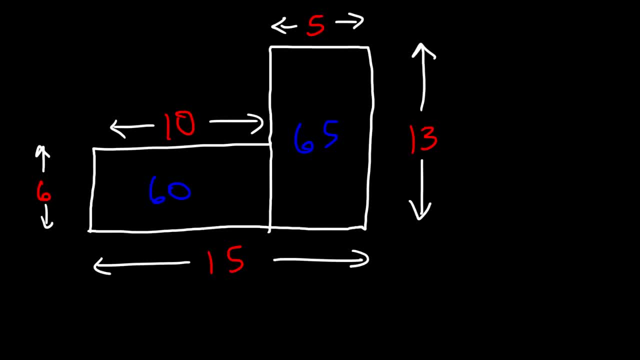 60. So the total area of the composite figure is 60 plus 65. So we have 125 square units. So that's how you can calculate the area of a composite figure using rectangles. Here's another example that we can work on. 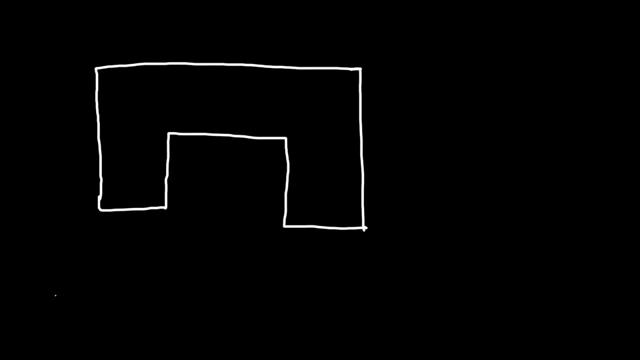 So let's say this side is 3,, this is 4,, this is 10, and then 6, and this is 11.. And let's say this is 5, and this is also 6.. So go ahead and take a minute and calculate the area of this figure. 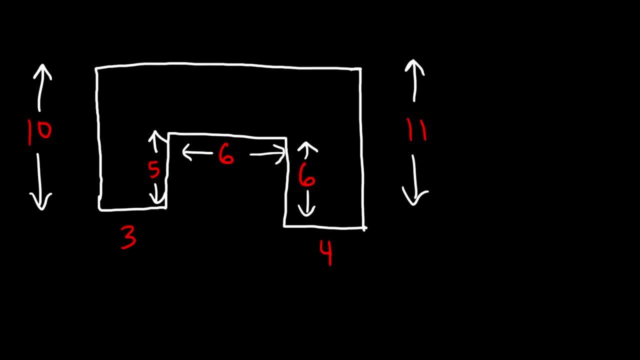 So how can we do this? What's the best way to begin? What I recommend doing is breaking it into three rectangles. So to calculate this one, it's going to be the length times the width, 3 times 10,, so that's 30.. 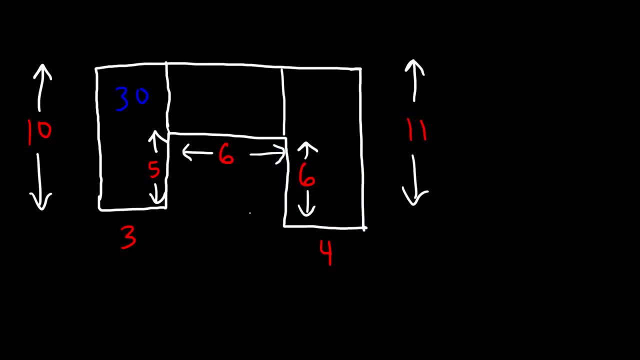 And then for this one, it's going to be 4 times 11.. So 4 times 11,, that's 44.. Now, what about this rectangle? It has the length of 6, but what's the? What's the width? 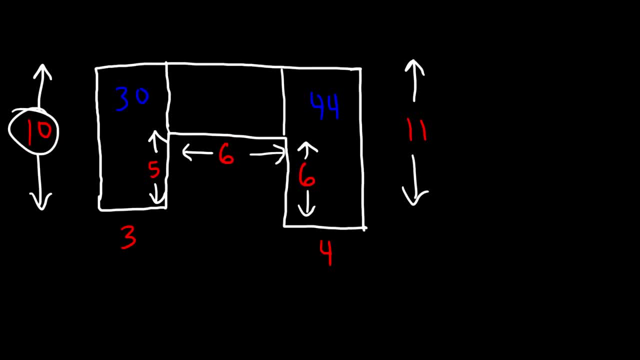 We could say it's the difference between 10 and 5, which is 6.. Or the difference between 11 and 6, which is That's 5.. Wait, this is supposed to be 5.. 10 minus 5 is 5.. 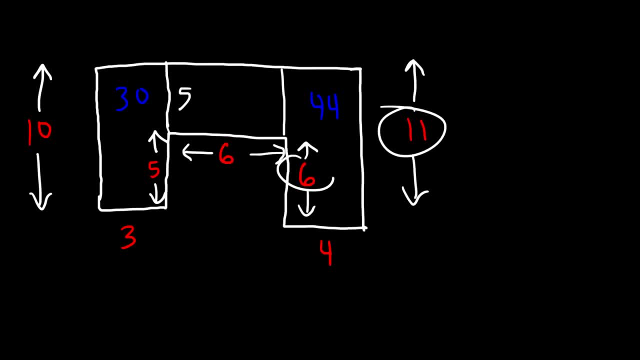 I don't know why, I put 6, for some reason, And 11 minus 6 is 5., So this is definitely 5.. So if we multiply 5 times 6, that will give us 30. And so this is the area of that rectangle. 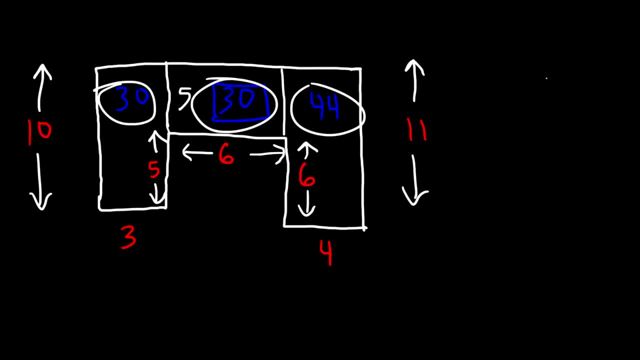 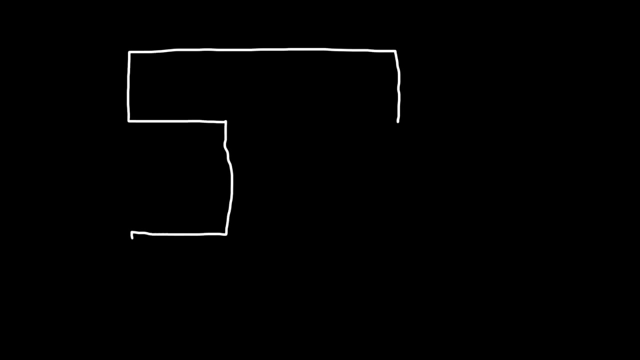 So now we need to add up these three values, So 44 plus 30 plus another 30. So this is going to be 104.. That's the total area of the figure. Let's work on another example Now. let's say that this side is 15.. 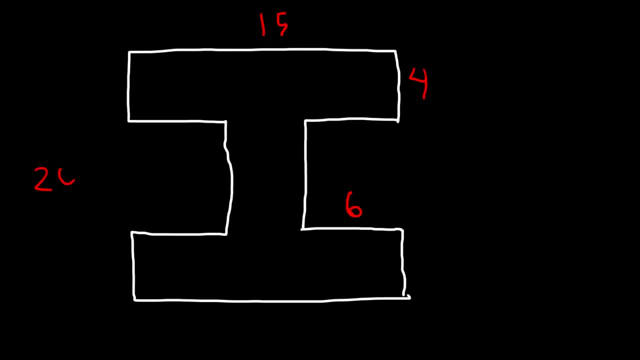 This is 4.. This is 6. And that's 20. And 19.. rep rules: Go ahead and calculate the area of this figure. If you want to feel free to pause the video. Now, let's say that this figure is symmetrical. 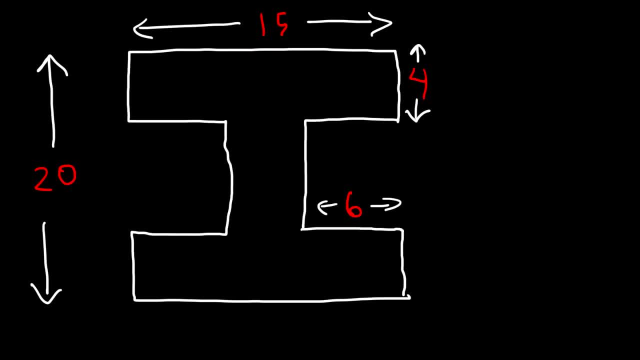 So that means that If this side is 15.. The other side is 15. And if this is 4, that's 4 as well, and if that's 6, then this side must also be 6. now, what about the length of this? 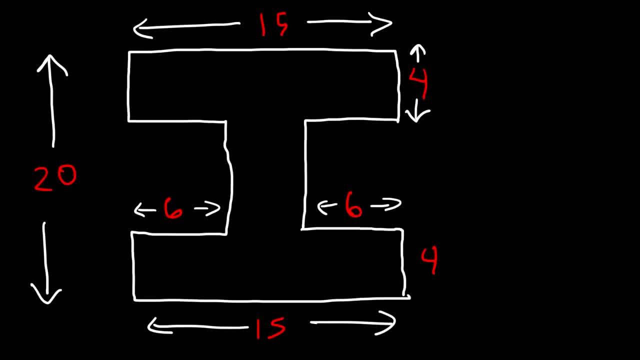 side. how long is it? so? notice that this side is 20 and this is 4 and that's 4. so it's the difference between 20 and 8. so 20 minus 8 is 12. so therefore, this side is 12 units long. what about the length of this segment? that's gonna be the. 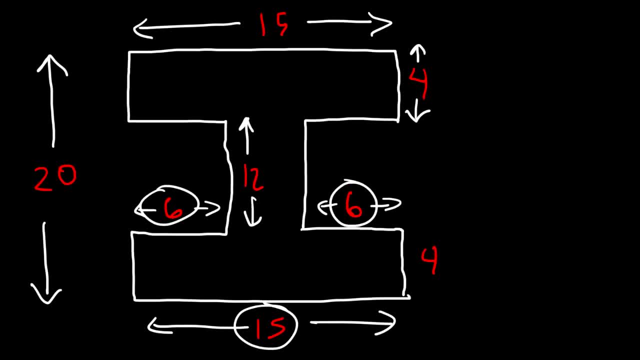 difference between 15, 6 and 6. 6 plus 6 is 12. 15 minus 12 is 3, so this part is 3 units long. so now we can calculate the area of this composite figure. so let's turn this into a rectangle. what's the area of the rectangle? so it's gonna be: 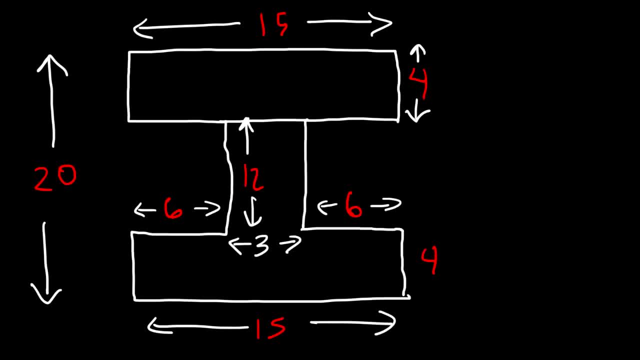 length times width, 15 times 4, which is 60, and that means that this part is also 60 as well. now to calculate the area of this rectangle, it's gonna be 12 times 3, which is 36, and so we got to add 60 plus 60 plus 36. 60 plus 60 is 120, 120. 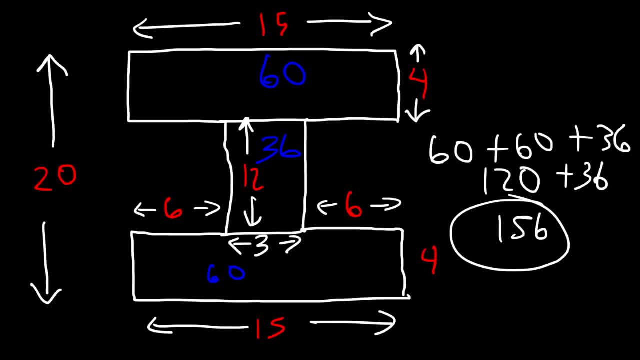 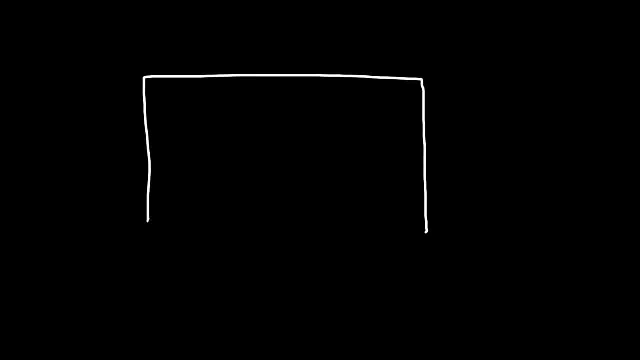 plus 36 is 156. so that's the area of the composite figure. now let's move on to the next problem. so let's say if we have a rectangle inside of another rectangle. now let's say the dimensions of the large rectangle. let's say it has a width. 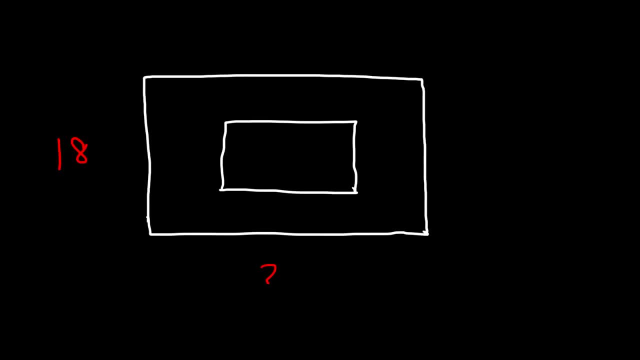 of 18 and the length of 25. now let's say the dimensions of the large rectangle. let's say the dimensions of the small rectangle. let's say it's 6 by 12. what is the area of the shaded region? go ahead and try that in order to calculate the. 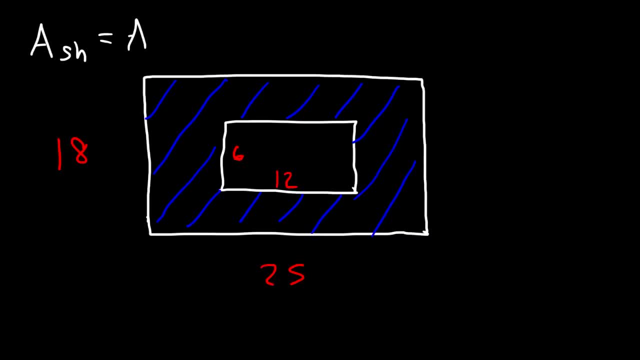 area of the shaded region. we need to calculate the area of the large rectangle and subtract it by the area of the small rectangle. so we're gonna do that with the rectangle. so the dimensions of the large rectangle is 18 by 25. so length times width, 25 times 18 will give us the area of the large rectangle. now to 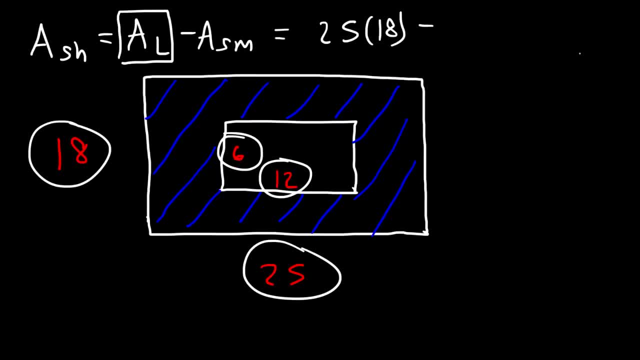 calculate the area of the small rectangle we can multiply the length and the width, so the length is 12, the width is 6, so the area of the large rectangle is 25 times 18, which is 450 square units, and the area of the small rectangle is 12 times 6, which is 72, so 450 minus 72. 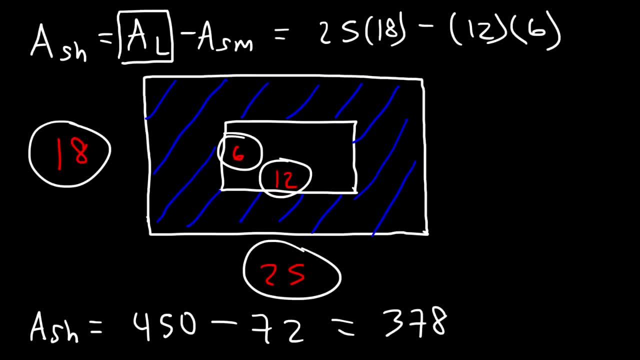 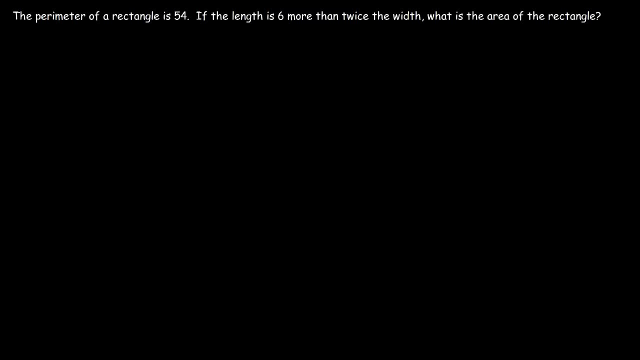 that's 378 square units and that's how you can calculate the area of the shaded region. it's the difference between the area of the large object minus the area of the small object. now let's try a word problem. the perimeter of a rectangle is 54. if the length is 6 more than the area of the large rectangle, then the area of the 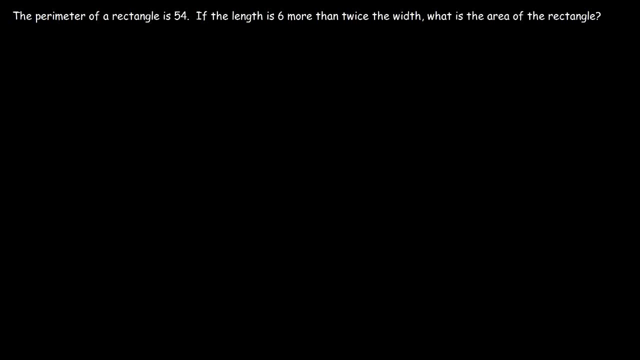 rectangle is 54, then twice the width. what is the area of the rectangle? so let's draw a picture. so this is the length, this is the width. the perimeter is the sum of all four sides. it's 2 L plus 2 W. so we're told that the 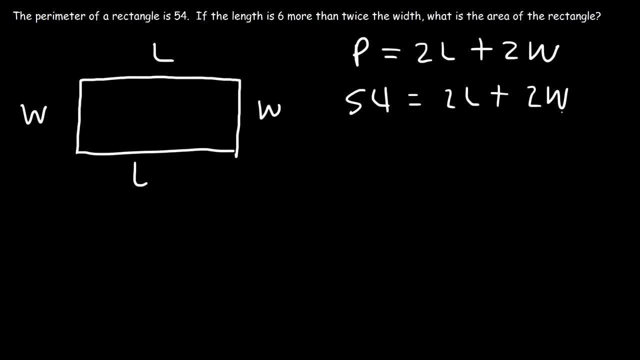 perimeter is 54. so we have this equation. now, to simplify it, I'm gonna divide everything by 2. half of 54 is 27, and then 2 L divided by 2 is L, 2 W divided by 2 is W. so we have this. 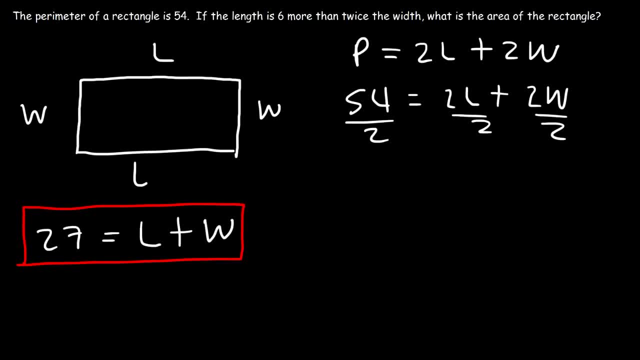 equation L plus W is 27. now we have two missing variables, L and W. so we need two equations to find L and W. now we're told that the length is 6 more than twice the width, so 6 more at 6 plus twice the width. so what I'm gonna do is I'm gonna 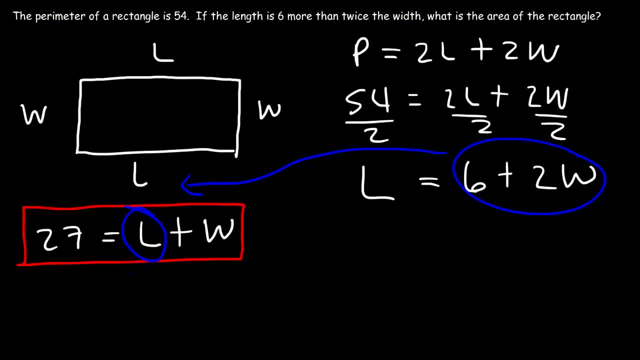 replace out with 6 plus 2 W. I'm gonna solve by substitution. so 27 is 6 plus 2 W plus another W. now we can combine like terms: 2 W plus W is 3 W, and now let's subtract 6 from. 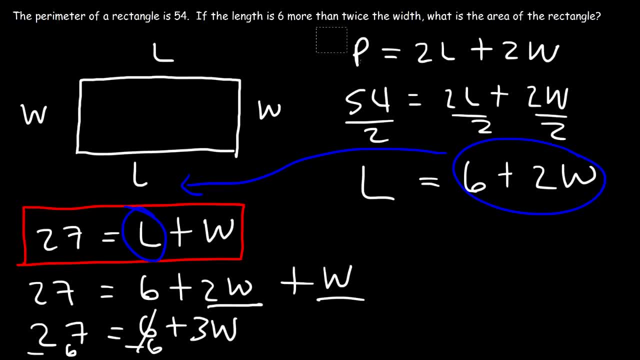 both sides, 27 minus 6 is 21, and that's equal to 3w. So if we divide both sides by 3, we can see that w is 27 divided by 3, which is 7.. So if w is 7, what's the length? So now we can go back to this equation: l is equal to. 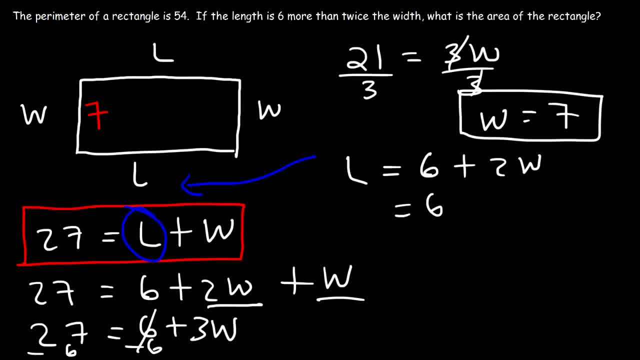 6 plus 2w, So that's 6 plus 2 times 7.. 2 times 7 is 14, and 6 plus 14 is 20.. So the length is equal to 20.. So now we can calculate the area It's going to be, the length.